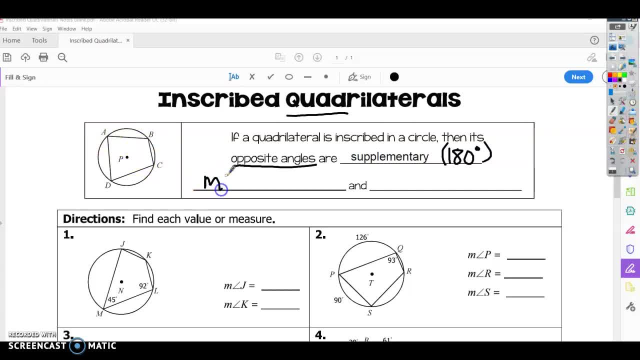 equal 180. So we can say: the measure of angle A plus the measure of angle C equals 180 degrees. All right, and the other two angles are also supplementary. So we can say: the measure of angle B plus the measure of angle D equals 180 degrees. 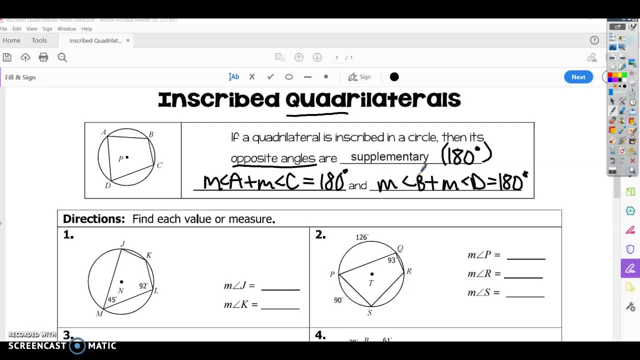 All right. if we look at number one, first example, it says: find each value or measure. Remember, when we talk about measure, we're talking about arc measure, or a value can be an angle, or sometimes it's even going to ask for maybe x. 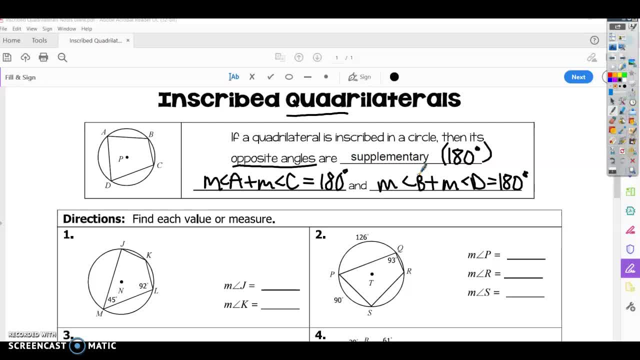 So for number one it says m is 45,, l is 92, and we have a four-sided figure. so we know we have a quadrilateral inscribed inside of a circle. so opposite angles add up to be 180 degrees. So k plus m equals 180,. 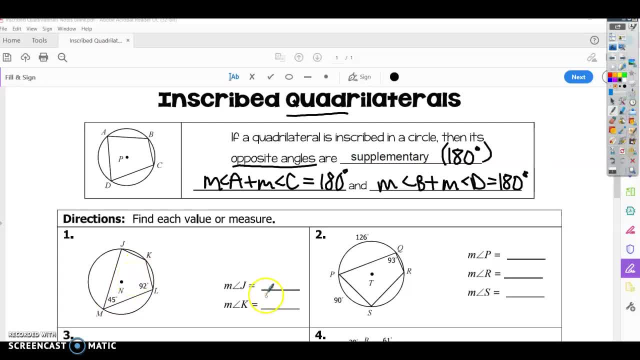 so we can do 180 minus 45 to get k, which is 135 degrees, And then 180 minus 92 gives us j, so that would be 88 degrees. All right for number two. it gives us one angle. This one's a quadrilateral as well. 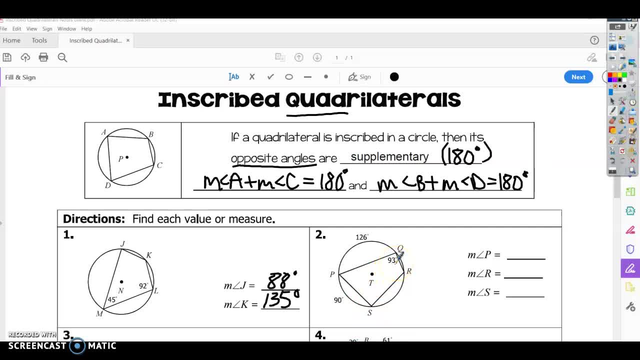 so we can find s by doing 180 minus 93, so that's going to be 87. And that's the easy one. So the other two are missing and they're opposite angles. So we have to think about what do we know? What did? 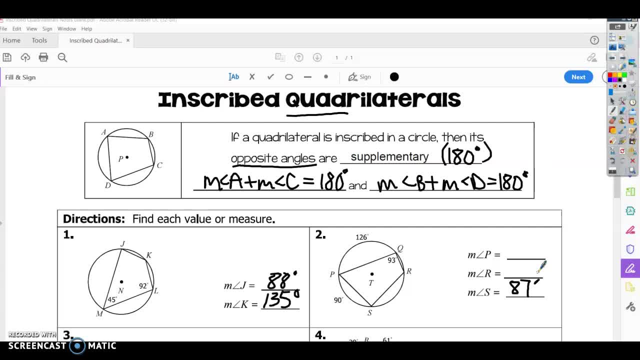 we learn before now. So we talked about inscribed angles before, so we're going to have to look at this. quadrilateral is different inscribed angles. So if we look at this angle here, we know that this arc measure from P to R is half the distance, or twice the distance of s. So we 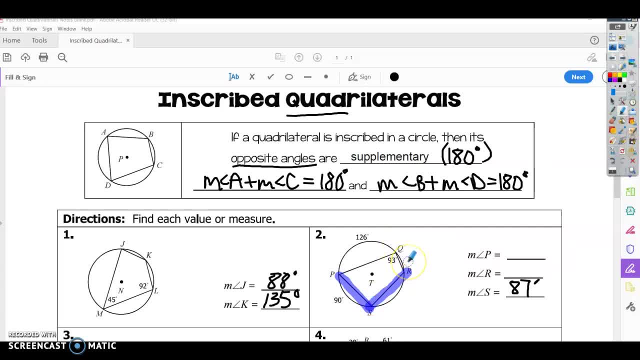 can find s using that if we can find this extra piece here, so we're going to have to find that piece. and another piece of information that we have is this right here, from P to Q to R. this is an inscribed angle as well, so the arc. 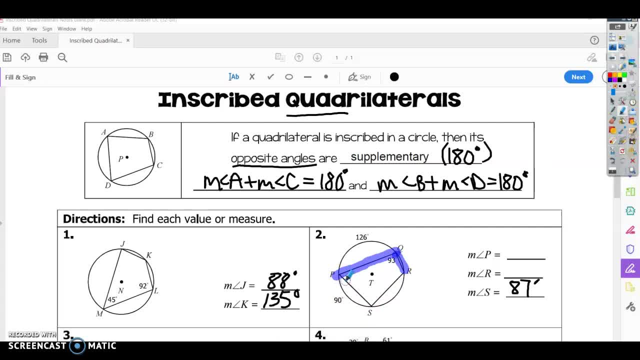 measure is double the angle. so if I take double 93, so 93 times 2 is 186, and then I already know part of that is 90. so subtract the 90 that gives me this piece here as 96, and then we can do 360 minus these three arc measures to get the 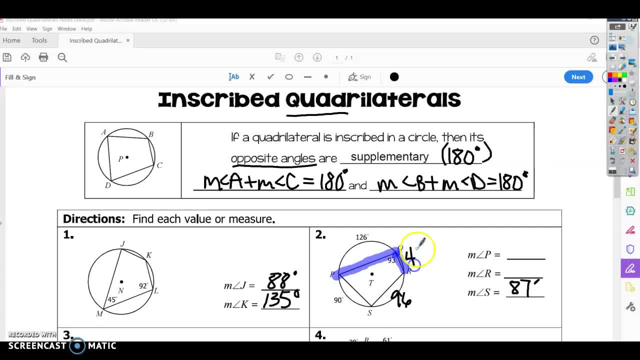 third, the fourth arc measure, to get the third arc measure, to get the fourth arc measure, to get the third arc measure, to get the fourth arc measure, to get the arc measure which is 48, and then we can use the arc measures now in order to 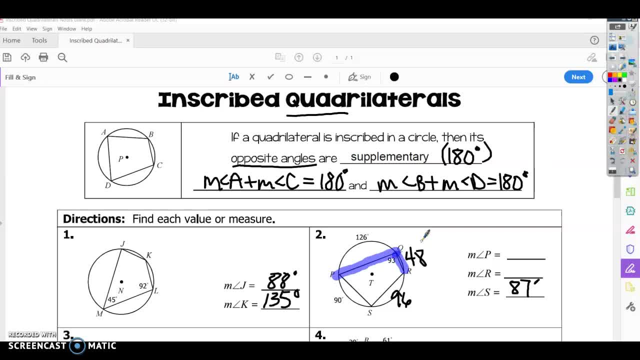 find the other two angles. So let's see what we have. So let me erase this here, Alright. so we need to see which angles we need, and we need P and R. So let's look at P first. So we need angle P so we can use this whole arc, which is 48 plus 96 combined. 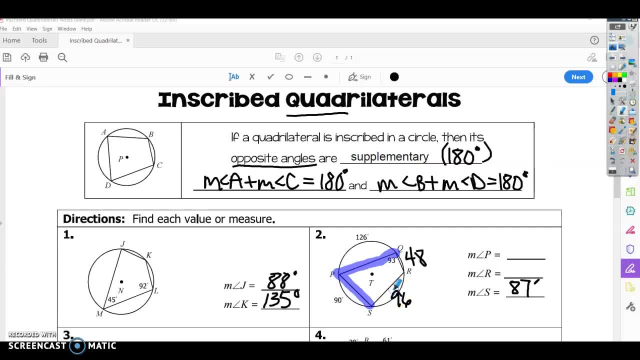 and we add that to the other TWO angles. So let's say this: third and fourth angles will add that up, and then we divide by 2, because the angle is half the arc measure. so 96 plus 48 is 144, and then half of that is 72. so this angle here is: 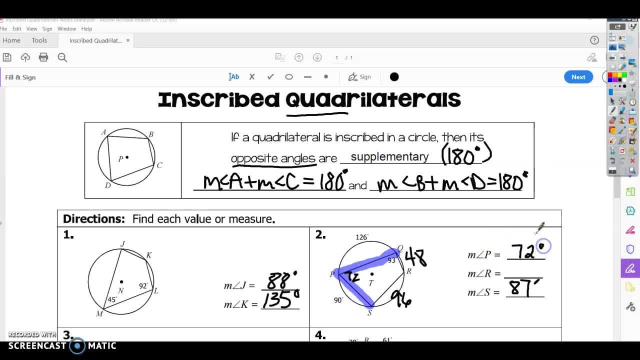 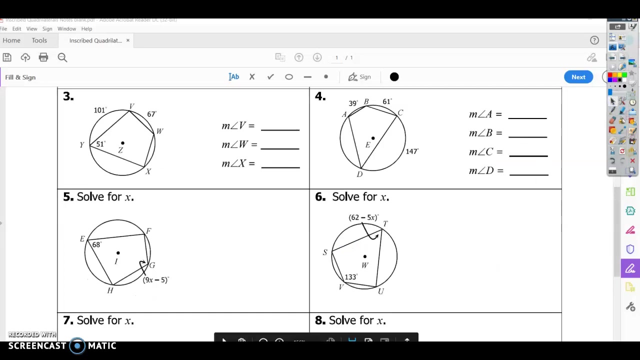 72, so that's P. all right, and then we're going to do the same thing for the other angle, or instead of doing that. now you know these two add up to be 180, so you can do 180 minus 72, and 180 minus 72 gives you R, which is 108. all right. 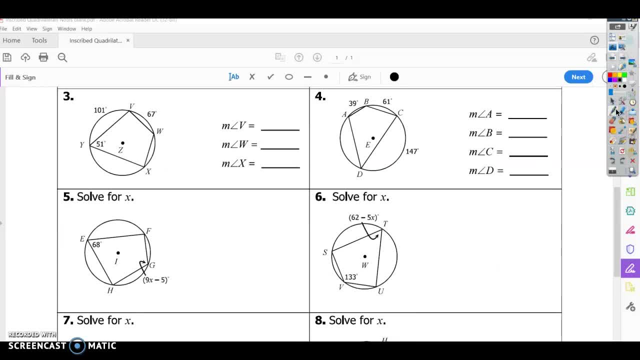 number three is an inscribed quadrilateral and again we only have one angle. so we're going to do 180 minus 51 to find W, and W would be 129, because those are opposite angles. and then again we're going to have to use the arc measure in order to find some of the others. so let's start with. we know. 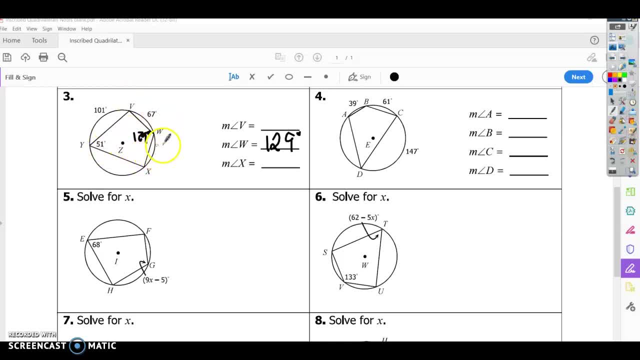 part of this arc, so let's find the rest of it. so to find this missing piece I'm going to have to do 51 times 2, which is 102, and then subtract 67, so that means this arc is going to be 35 and then. 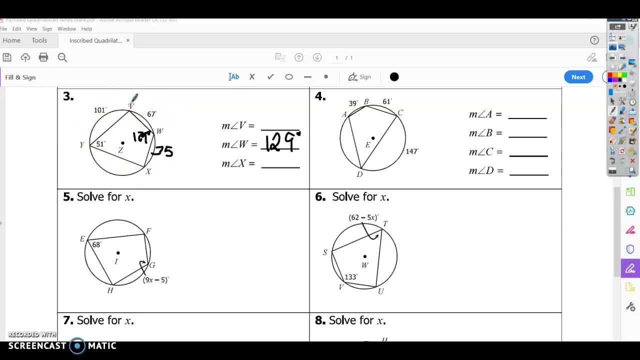 extra 3.32 minus 167 minus 35, that means this part is 150, 27, 167 down the rate. aquest Jeune Vaillant 12ender 1370 eli going to have to use an arc measure to find one of the other ones. So let's look at v. So v is. 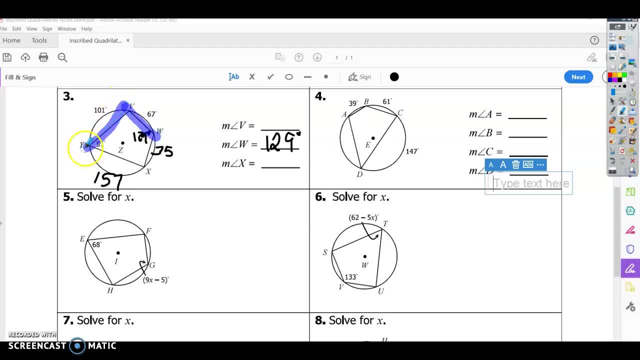 this angle here, and that means from y to w, is our arc measure and we know this is twice what the angle is. So I'm going to do 157 plus 35 and then divide that by 2. So 137 plus 35, 157 plus 35. 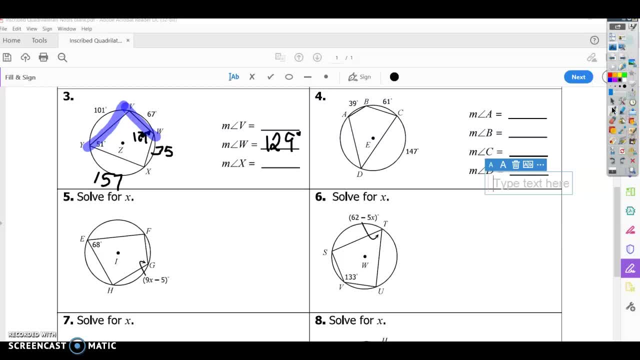 is 192.. 192 divided by 2 is 96. So this angle v is 96.. Then we know that 180 minus 96 gives us x, so this one is 84.. All right, number four doesn't give us any interior angles, so we're going to have 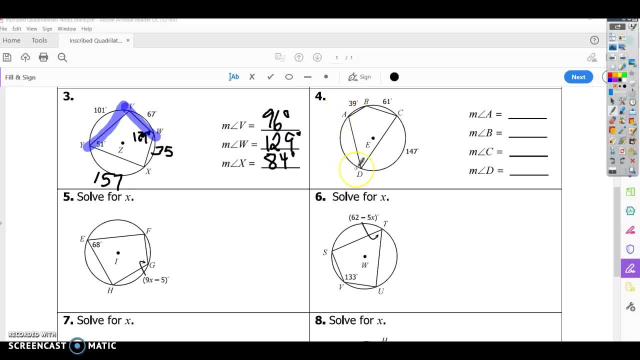 to first figure out what our arc measure is. So do 360 minus these other three arcs, and that's going to give you 113 for this arc measure. now we have all the arc measures and we can look at one angle at a time, so just choose one, it doesn't matter. 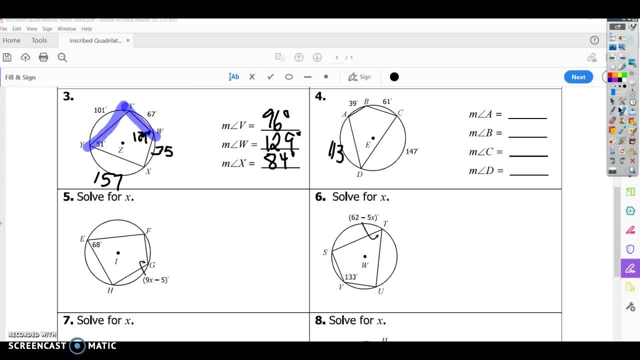 which one you start with. you know that an inscribed angle is going to be half of the arc measure, so maybe start with angle b. okay, that means this whole arc from a to c. so that's 113 plus 147 is 260, and so b is going to be half of 260.. so divide that by 2 and you get 130. 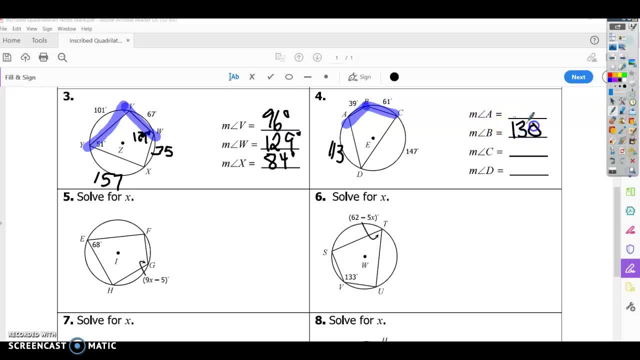 so angle b is going to be 130.. so this one's 130.. we know, together these two are 180. so you can easily find angle d. so angle d is going to be 50.. all right, now we're going to have to look at a different angle to find, or a different arc to find. 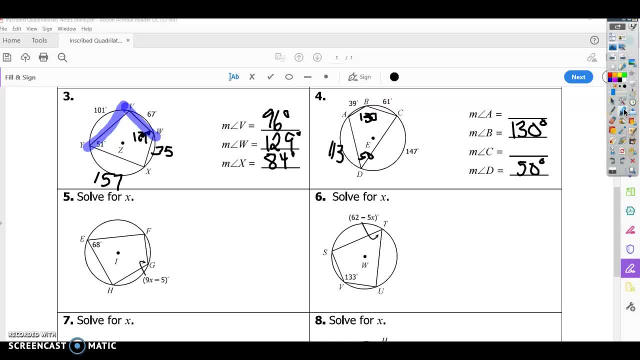 another angle. so we need to find either a or c. so if we look at a, here's a, so it's two sides go from here to here, so it's going from b to d. so i've got 61 plus 147, and then i divide that by 2. 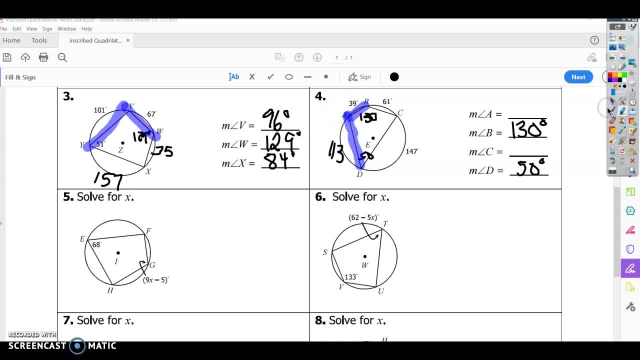 work this out first, or y, and i divide that by two. so here's the first side. all right, so angle b is going to be four and angle c is going to be four and angle d, w is going to be four and angle d is going to be four. 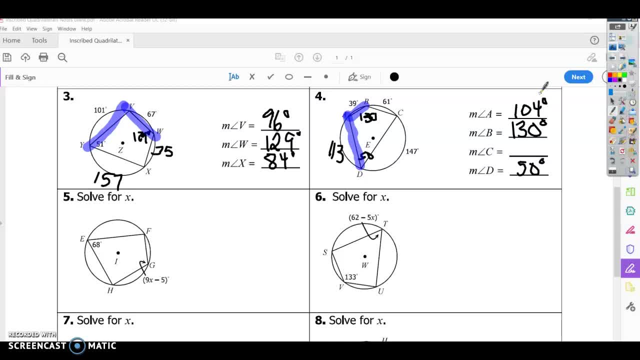 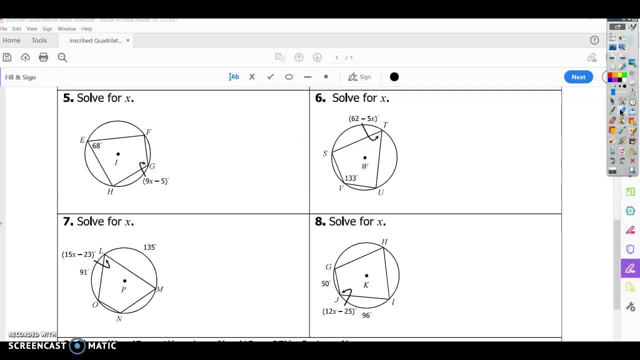 and angle c is 1 over square, which isля d plus 50 is 104.. so angle a is going to be 104, and then 180 minus 104 is 76, And this angle equals 9x minus 5.. So we can say 9x minus 5 plus 68 equals 180, because opposite angles are supplementary. 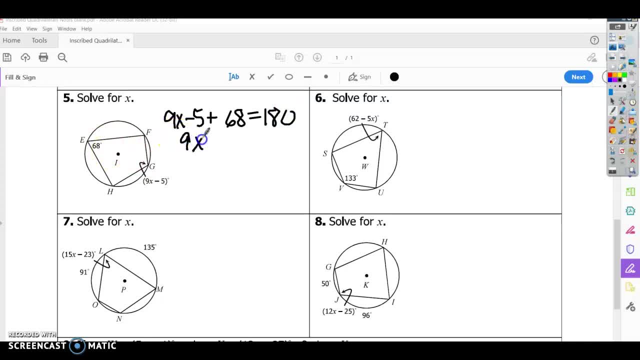 So they add up to be 180.. So I've got: 9x plus 63 equals 180, subtract 63, 9x equals 117, divide by 9, x equals 13.. All right for number 6, it's going to be very similar. 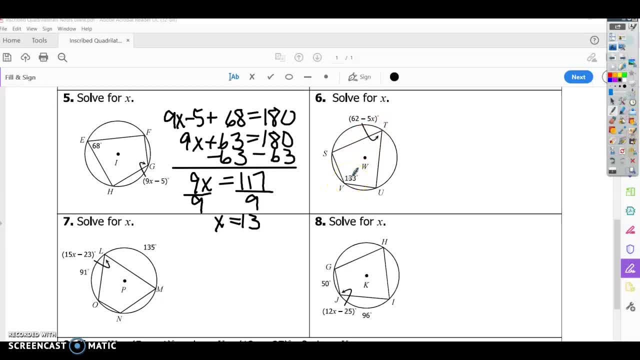 So we've got opposite angles. They add up to be 180. So I'm going to have 62 minus 5x plus 133 equals 180. And then I've got negative 5x and I can combine 62 and 133. 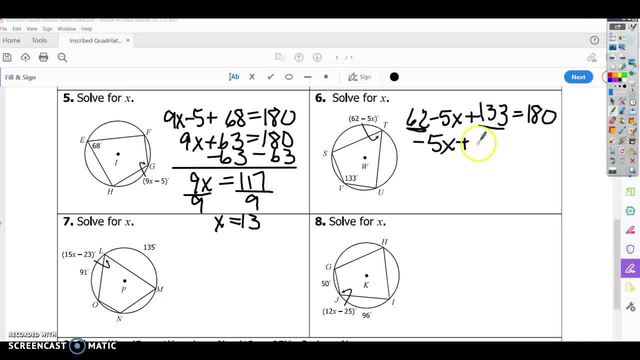 They're on the same side. So that is a plus 195, and that equals 180.. So subtract 195.. Again, we're solving for x, trying to get x by itself. 180 minus 195 is negative 15.. 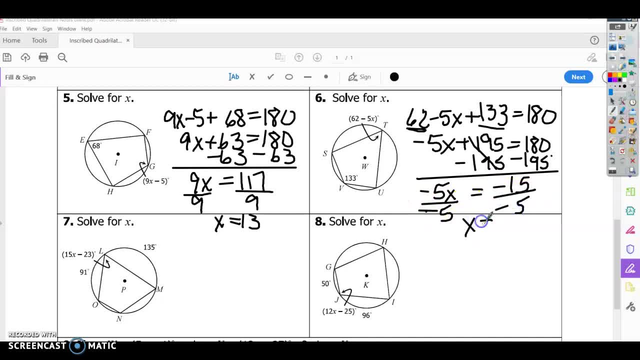 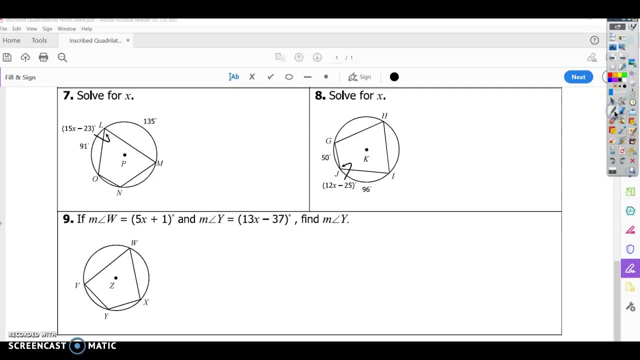 Divide by negative 5, x equals 3.. All right, and this time it said solve for x. This said solve for x. All right, number seven says solve for x, and we know that these two angles add up to be 180.. So this one. 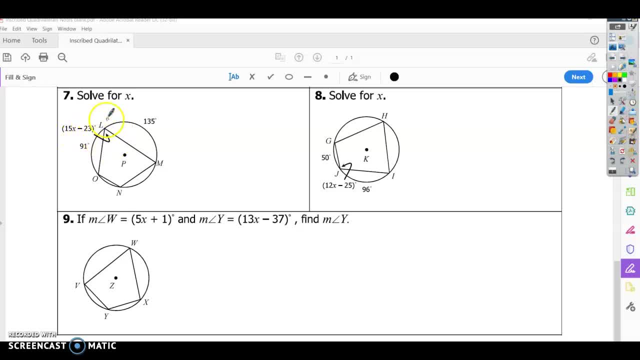 it gives us this value 15x minus 23 for l and n. we don't know, but we can find it because if we look we have an inscribed angle and we know both of these arc measures. So 135 plus 91 is 226. 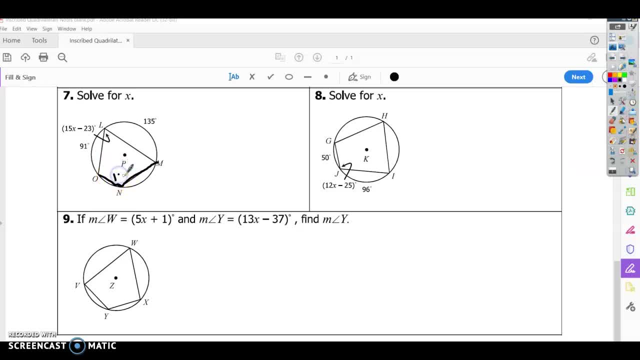 and the angle is half of that. so this is 113.. All right, so we're going to have 15x minus 23 plus 113, and we know these are supplementary, so they equal 180 degrees. All right, so I'm going to have 15x. if I do 113 minus 23, that gives me. 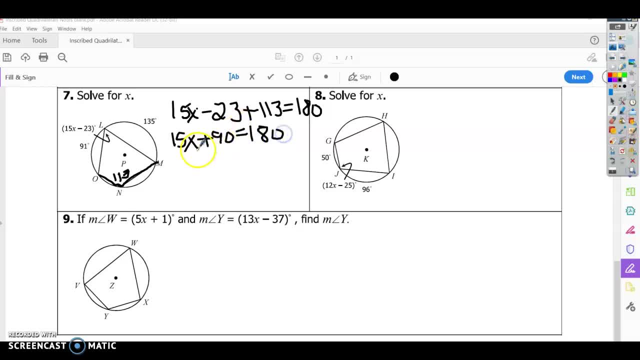 90. I'm going to subtract 90 from both sides and 15x 180 minus 90 is 90. So divide by 15 x equals 6, and this time it said: solve for x, so x equals 6.. You can also plug that back in 15 times.